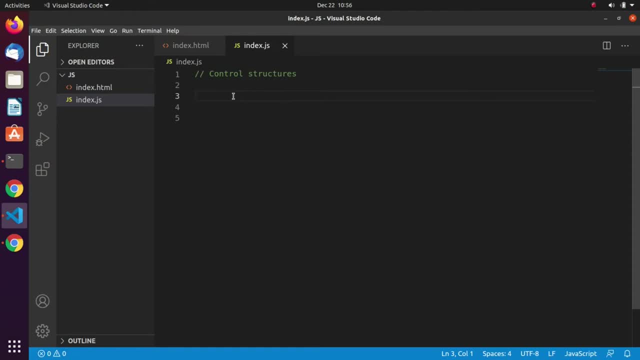 code, okay, enclosed within braces. so the structure provided by the use of conditional statements utilize the booleans to determine whether or not a block gets executed. so in this use of booleans, any defined variable that is neither zero nor an empty string, will be evaluated as true. okay, so now let's talk a bit about the 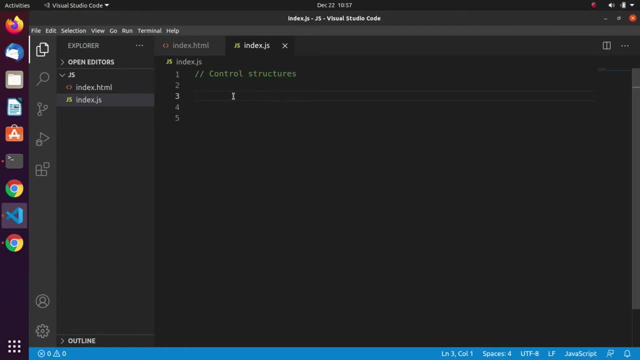 if, okay, so the if, the if statement is straightforward, okay, it's very straightforward. so if the given expression is true, the statement or statements will be executed. otherwise, a skip. okay, so we have. if you take some condition, okay, so we have in. if something, then do something. okay, so you. 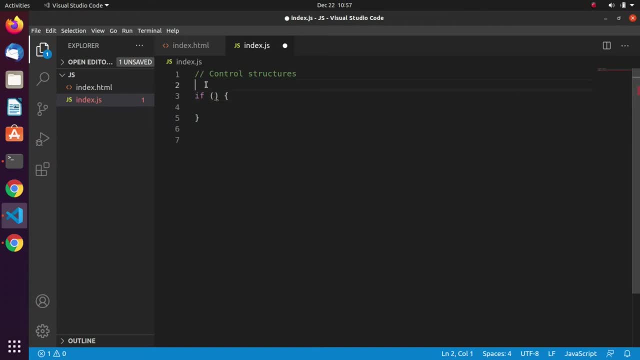 can tell, if I'm just declare a variable caller X equals to four, okay, and then a variable y equals to like eight, let's say okay, something like this, then i can just say: if y equals to x, then do something. i can just say: document dot write. 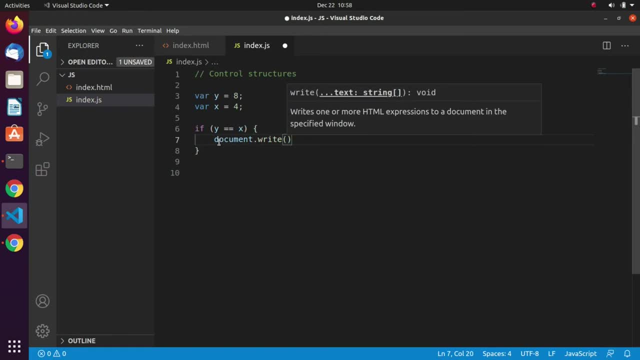 it great or something like true. okay, remember from our previous tutorial we saw something like this: so that's how the actually the if actually works, okay, so you just check. is, as we said, this straightforward? okay, the first check is this: is y equals to x in only data, not the type? okay, 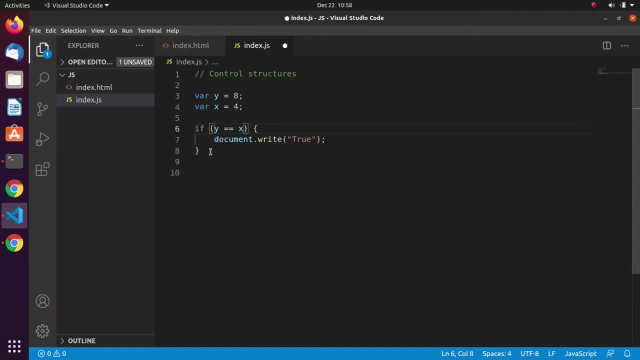 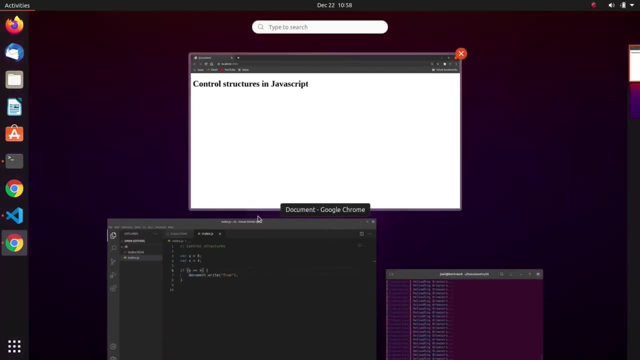 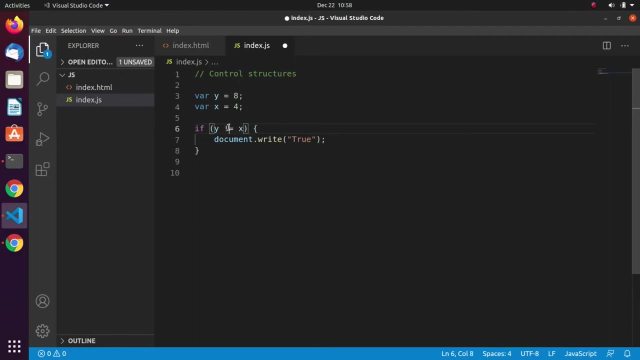 so remember, the double equal, not the triple one, okay? so if it's the case, then true, let's go ahead and see what it shows in our browser. you see there's nothing there, because actually x is not equal to y. okay, but let's take for a. 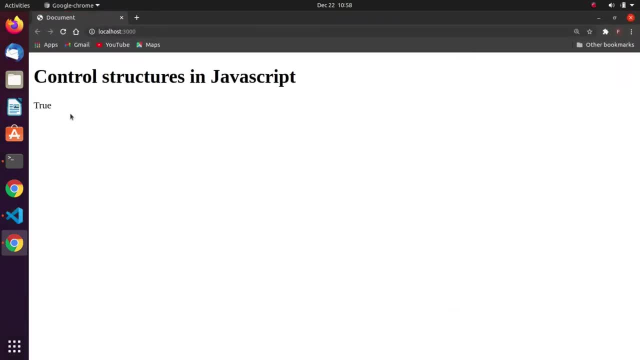 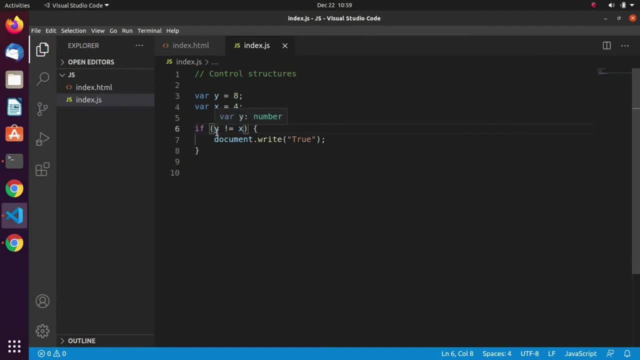 difference. okay, it's h different from y. then you see, here we have true. okay, so how. that's how the if actually works. so the if statement may also consist of multiple parts, incorporating else and else, if. okay, these keywords are part of the if statement and identify the code. blocks of that are executed. 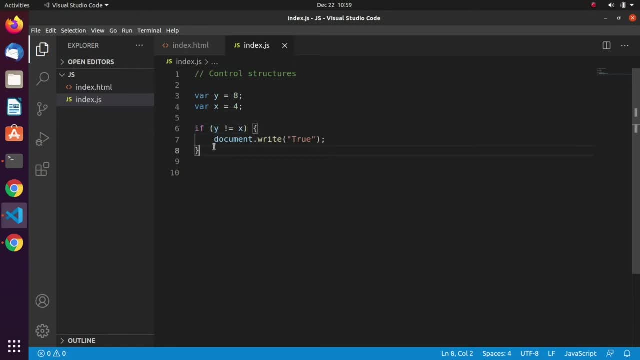 if the precision considered condition is false. so that means, if it's not the case, you can have something like else. if, okay, if something, that is, if that first condition is false, then try to check this one. maybe it will work. or if not, then maybe we should skip, and then it's going to be false. 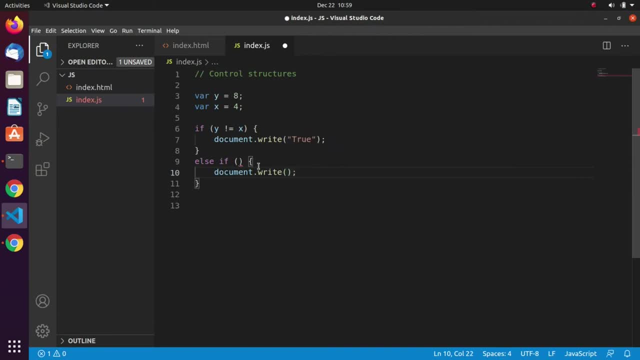 again. i'll write something like this: okay, so that is, if else, if what? you can just check: if y is instead greater than five, okay, here i can see if y is equal to x, and then here i can say: if y is greater than five, then right, y is greater than five. okay, so you can put it else. 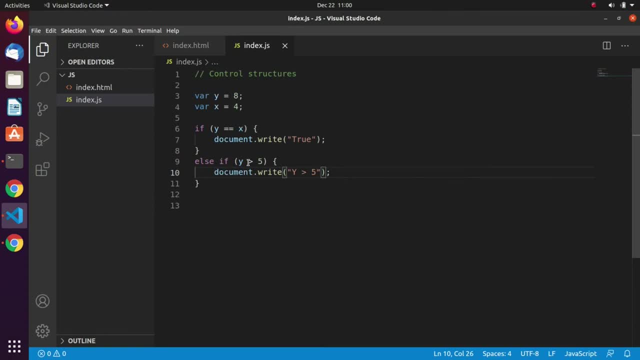 if notice, if this one is not true, then try this one. if it's not true, you can of course change many else. if else, if okay, there's no problem with that. so you can just do something like this, and then i'll write some code here contain, and then finally you have an else that. 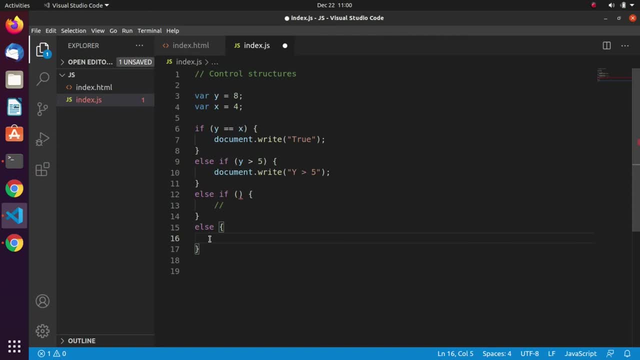 means if none of above okay was true, then just jump into this. that's how the else the if- actually works, so only one within this, either this or this, or this or this, will be executed. not all okay, not all. so when one is true, no matter the remaining one, then you just do the first one and then skip the. 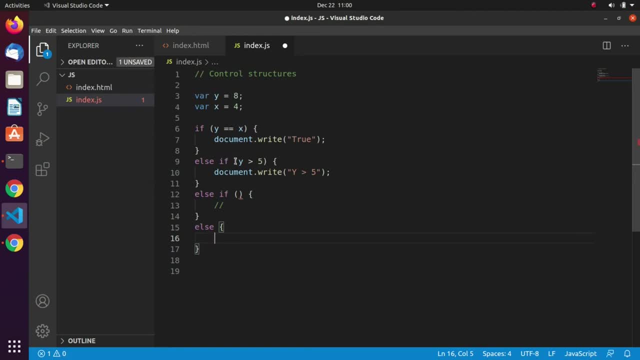 second one, if it's true, but normally it should not be. you cannot put two conditions that okay. that should be satisfied to confuse the accurate. but if you want to do that, you can still use if something like this: if do this, okay. and if you want to check another condition independently from the previous, 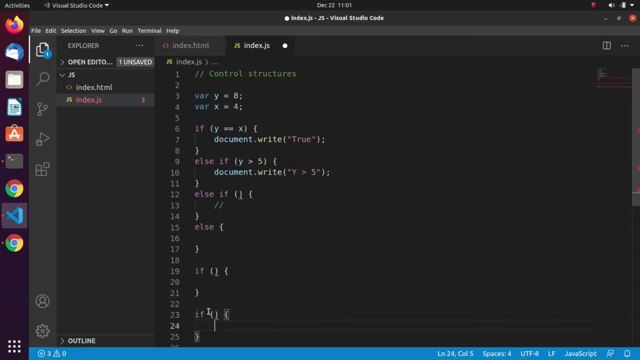 condition. you can just do something like: if again, okay, like this, separately, okay. if to this, if again, do this, and so on. so i hope you got the point from. for the if, let's go ahead and talk a bit about the why. okay, we also have the while, all right. 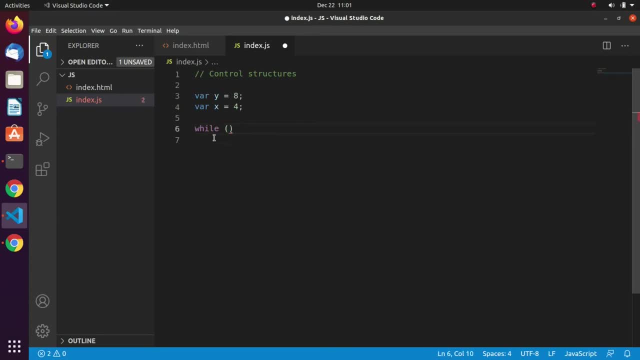 you have y and then something sorry. okay, why something like this y? maybe i can just say y x is greater than four. let me just say y, x is greater than eight or less. since x is okay, y, x is less than eight, then you can just do something there, okay. 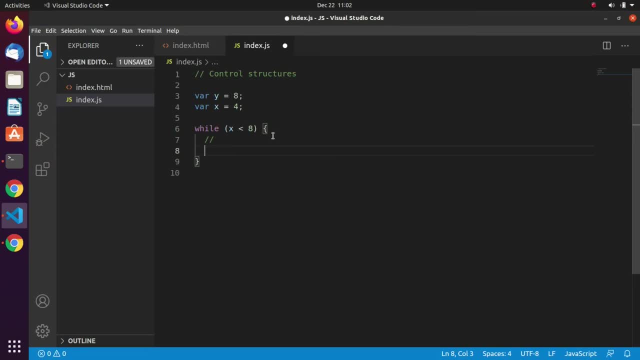 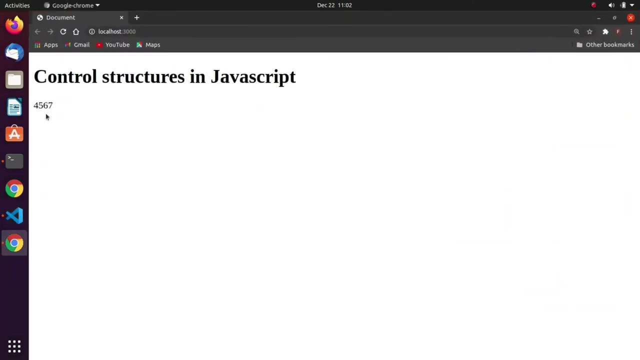 do something and then you can maybe increment. okay, say like x plus plus. all right, so let's do something like document dot write can just print the value of x. okay, let's go ahead and see what it shows. you see, here we have four, five, six, seven. of course it's just. 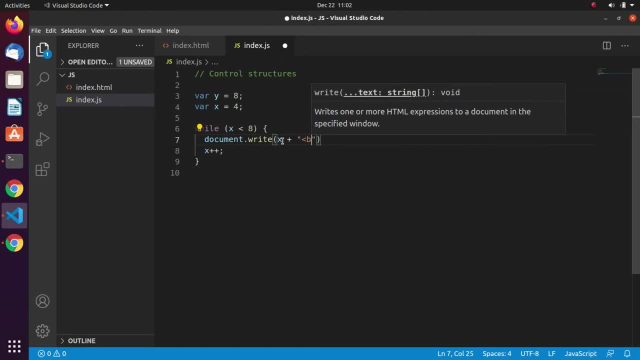 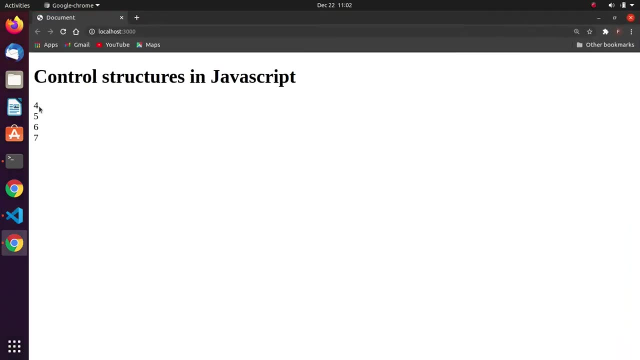 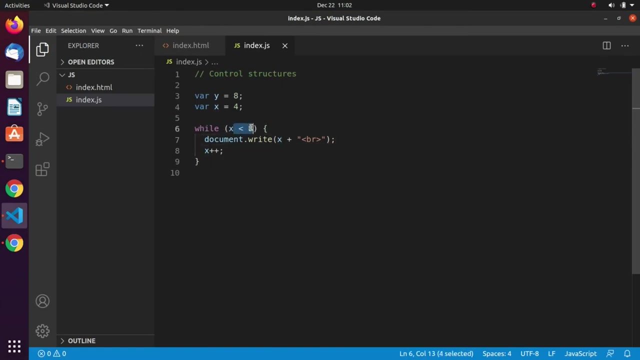 put everything at the same place, because there's no something like a break line and just put a break line there. okay, of course we have this. you see, here you have four, five, six and seven. so what the white actually does is what it takes, while this condition. 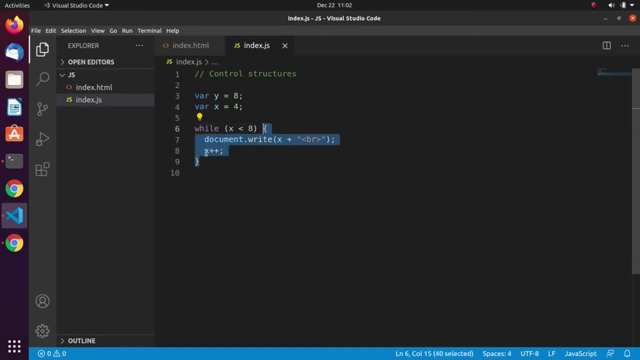 is true, just do what is inside between these codes. okay, this is braces. all right, so we print this and then we increment x by one. remember this operator from the operator tutorial. okay, so that's how the the y actually works. so that's how the y actually works. so that's how the y actually works. 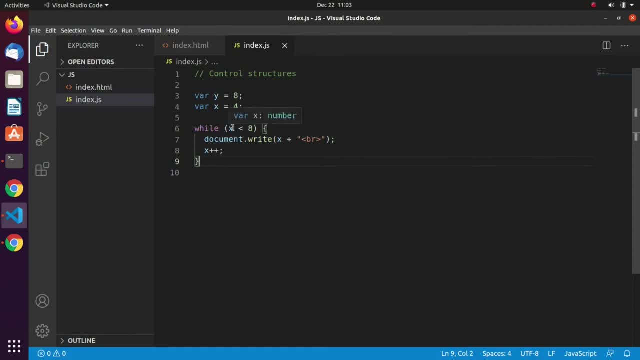 okay, we have also, so it will be incremental. xu becomes something like it: if we check, is it less than 8? no, you just go out of the loop and then continue executing the program. okay, so we have also the do y. okay, so now they'll do while. how does it work? okay, how does it work? so we have to do what actually do. 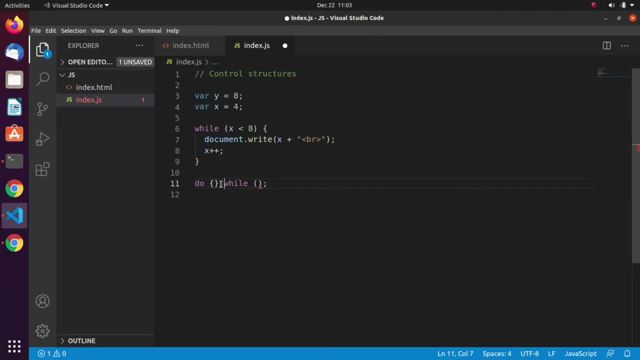 like this: okay, so we have some condition here, you have a code here and any condition here I don't know. you can go to: the X is less or equal down, why? okay, and then we have a code here. so the difference between the do white and the 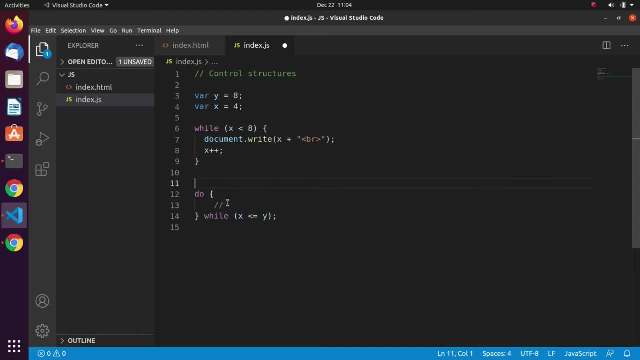 word is that the new execute at least once before start checking the condition, but do while they take the condition first before executing anything. but the do execute once, at least once before start checking the condition. so that's the only difference. okay, now let's talk about the four, but let's assume within 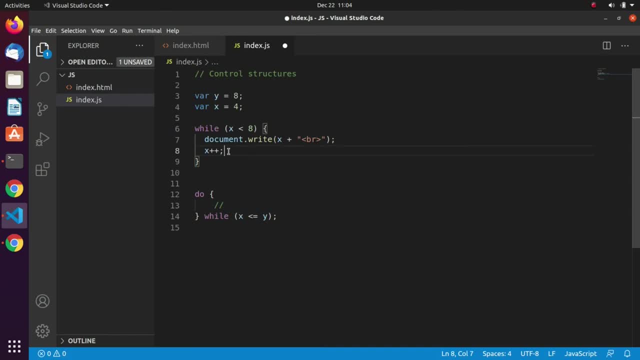 the loop, okay. or let me just say: let's see the four before I'll show you something. okay, tell you something. let's talk about the four before, okay. so for the four, you have four, and then we have three things, okay, to manage. first, the first thing is: 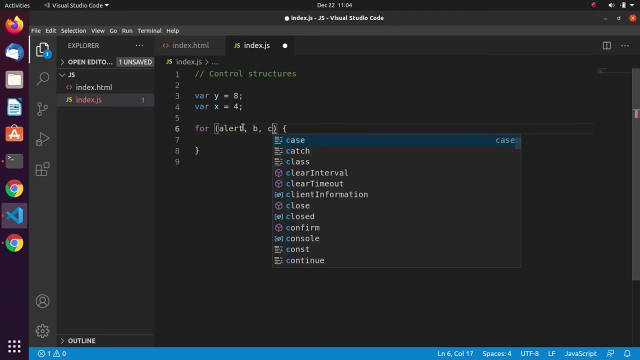 let me just put a, B and C. okay, so his name this: a- okay, is an expression, which is actually what? the initial expression, the B is the condition and the the C is the final expression. okay, let me just put something like: just go for practice and then put something. usually. 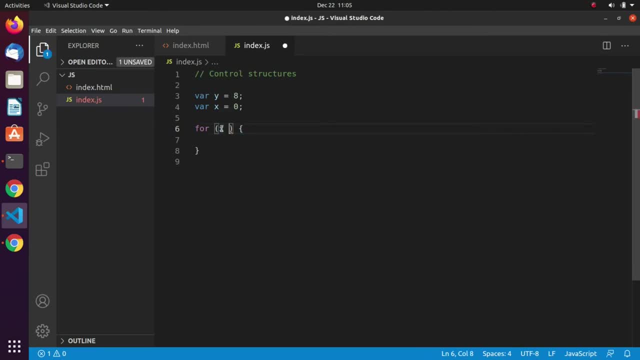 full there something explicit. okay, can you see X from zero? so I can just even declare X here like this, and then just say like this: where X is less than can just say 7, then increment X, okay, and then of course we have a code here now. 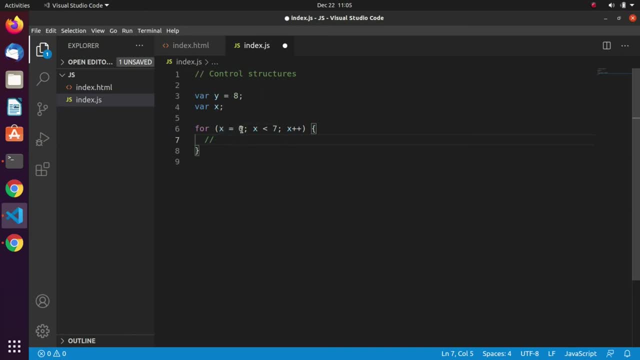 this means for X. that is the initial condition. X starts from 0 and then, while that X is less than 7, continue and be incrementing X. okay, till this condition fails, and then we go out of the loop. so that's how the for loop actually works. 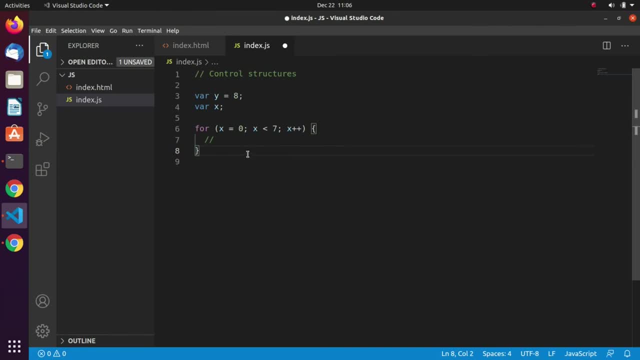 but the difference between the for loop and the Y. you see that the difference there is: the for has a limit, as you can see there, but the Y, okay, you can like set the limit from the for, but the Y is like it goes and then goes, goes, goes till. we don't know where to reach till. 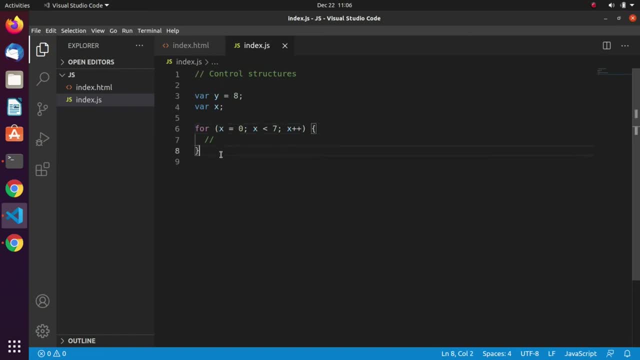 where something can happen, okay, and then maybe we can have something like: let me just show you, we can have Y one. this one is all sometimes very useful for infinite loop, so this Y one will mean it means that you can have Y one. this one is sometimes very useful for infinite loop, so this Y one will mean it means that 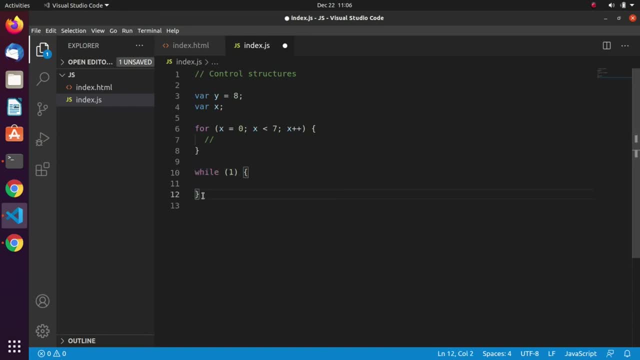 be executing this for a while. that is forever, okay. but of course we have to break somewhere. so to break, let's just use the keyword break. so this means execute something infinitely till something happen. when that thing happen, then just write this break keyword. okay, so we see the difference between the. 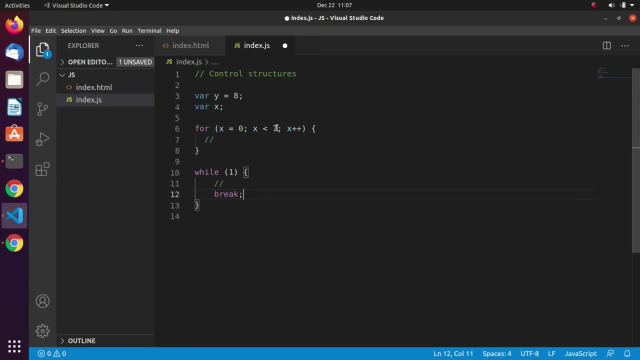 four. so with the four here we have a limit set, set to 7. okay, so this break. actually, of course, you can still use the break within the four. okay, so they do till maybe something fails. you just want to break. you don't more want to continue with the loop. you can just use the break keyword. okay, you. 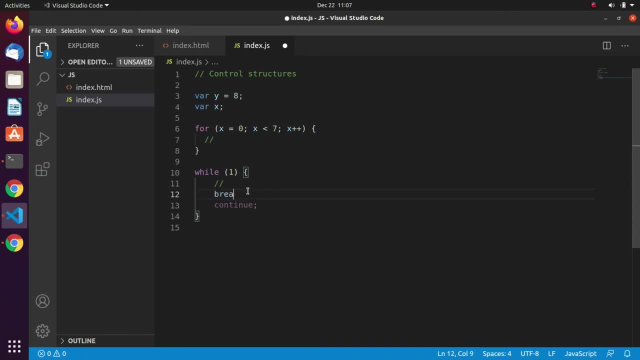 also have to continue. the continue is to keep to skip. to skip one operation- okay, maybe you are doing something and some, at some place you want to. something is not okay, you just want to skip, you don't want to execute it, okay, so that's what they do. 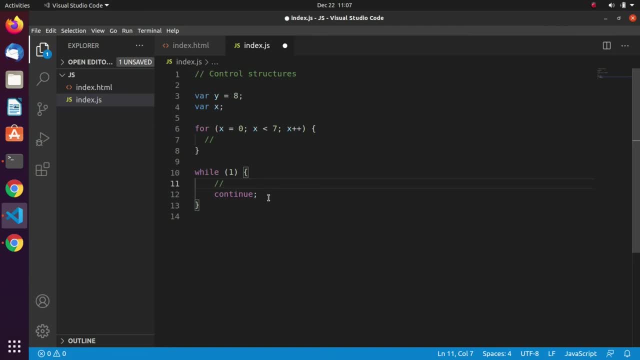 there's the continue operators, actually those keyword, okay, so I hope you got the point from that also. we have the switch, okay, the switch operator, so we have switch, then you're going to switch on what, and then we have cases. okay, we have case one, then case one, then do something and then break. okay, it's very. 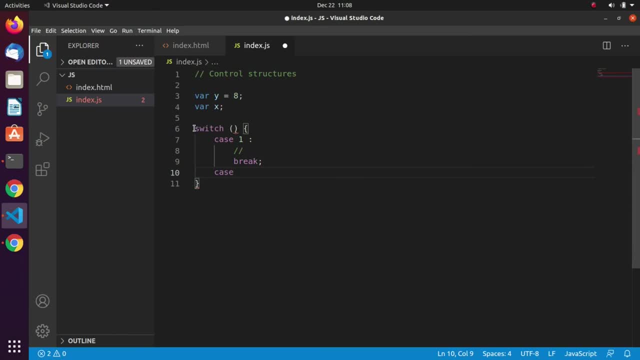 very straightforward. and then we can have case two and then break again. let me just put something here: we can break on the value of X. okay, that is X, so we have case two. and then we have something, execute something and then break. okay, so that's how do you, and of course we have the G for let me just do it and then 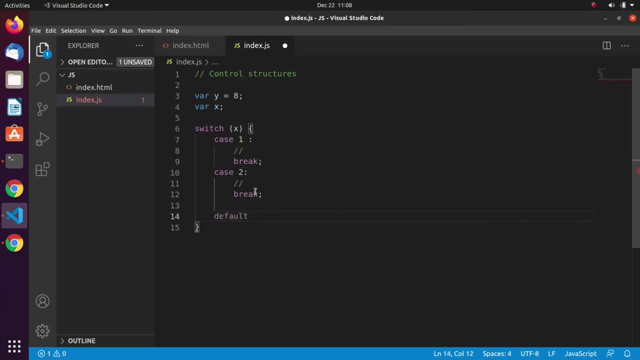 explain it to you and then execute something and then break. okay, so that's the structure of their switch. so what it does is that first it takes a value- okay, as parameters here to take on it. okay, to work on it. okay, the first trick: if x is equal to one, then do something here you can. 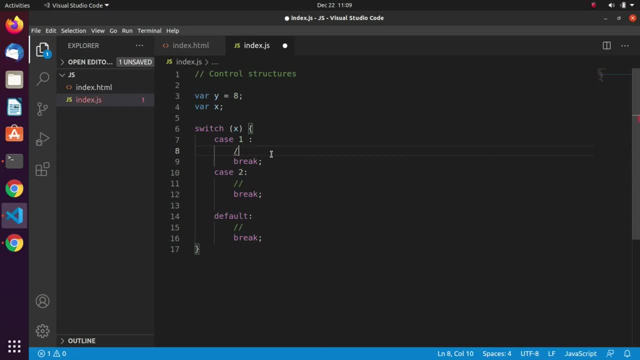 have any code here. okay, kind of write anything here, even on multiple link, so there's no problem, you can do something like that and write everything. okay, oh, you got the constant what I'm trying to stay here. so if x equals one, do this and then break, let it go out of the switch. but if 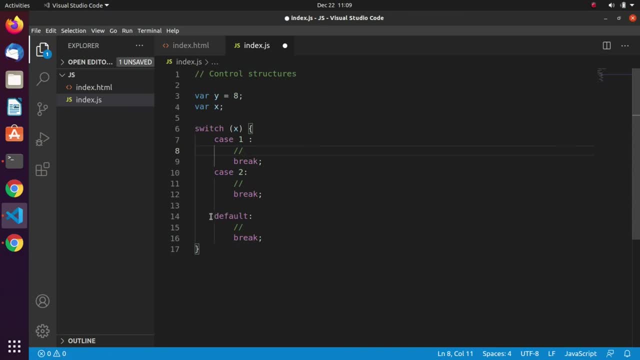 equals to two, just do something and then great default. if x is not neither one or two, then just go to the default and then break. okay, and now the break is very important, even though it seems strange that if one is, if X is one, you execute and if you don't put a break, you. 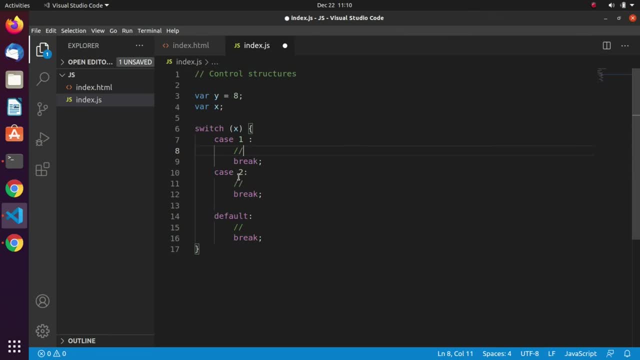 will then continue. if you don't put the break, you will take even the case of X equals to 2, even if X is not equal to 2. so it's very important to put the break after the the execution of what, any case, so you can have many cases as you want. 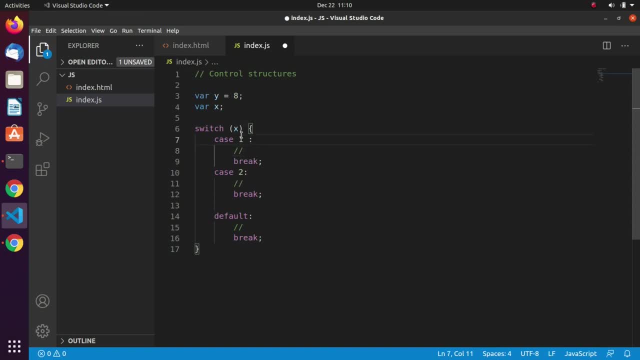 so there's no problem with that. okay, of course, we can even have a strings, so like something like you can see: if X equals to, okay, so we can do that on anything. okay, you can have a P and something like that. okay, just to explain you. so we are actually working with the value of X, based on that value. so this: